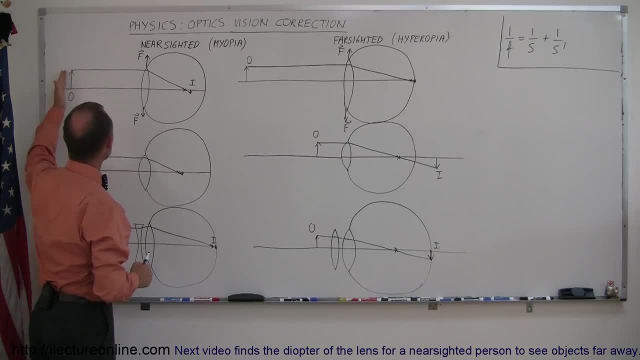 why the eye needs to do that is because objects that are very far away will form an image very close to the focal point, just right behind it, And if the focal point can be put near the back of the eye, where the retina is, then the image will not form on the retina, It will form before the retina, and so the rays that then reach the retina will not be very focused and the image will look fuzzy. Alright, so the objective then is to get the focal point to be further back, But the only thing the eye can do is let go of the focal point. 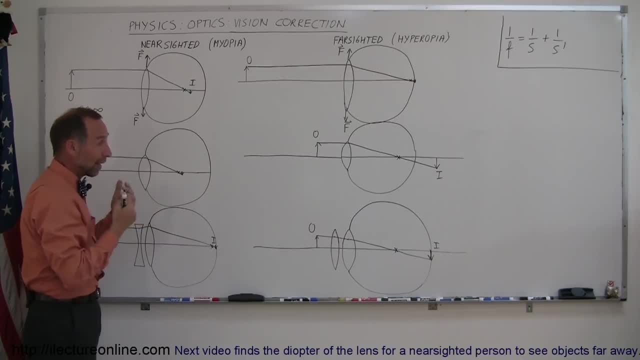 On those muscles, for example, and we do that involuntarily, We don't need to try that, We don't sit there and try to exercise the eyeballs, just naturally. So if we relax our muscles in the eye, then the eye will bulge up naturally, But then all that does is bring the focal point even closer, which means you can see even worse objects that are far away. Matter of fact, this is what we do when we want to see things close up, because when objects come closer, that automatically cause the image to fall farther back. 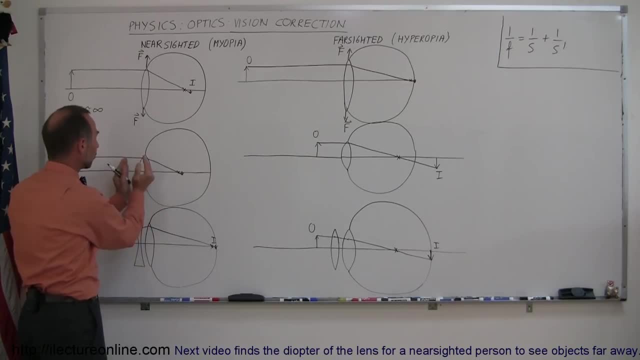 Away from the focal point, and so the bulge in the lens brings the focal point in and allows an image of something that's close up to form at the back of the eye. So if a near-sighted person, the farthest back that the focal point can be is in front of the retina and not far enough back, there really isn't anything else that person can do. 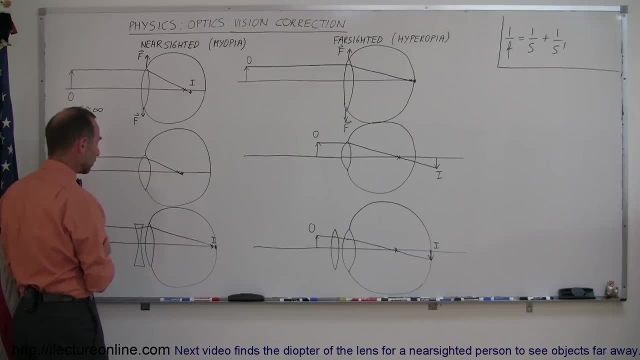 So the only thing left to do is put a corrective lens in front of the eyeball, and of course, that's not typically what the lens looks like, But I just wanted the shape of a diverging lens, because that causes the rays to diverge a little bit further, causes the focal point to fall further back, and then an object that's far away can then form an image right on the retina, like that. 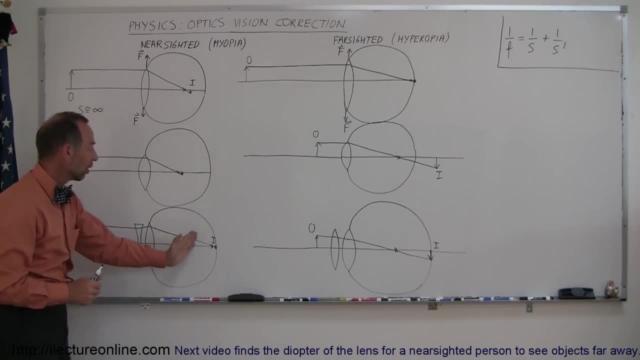 So that's why, when you're near-sighted, you need a diverging lens to put the focal point further back, so an image can form clearly on the retina. when you look at things that are far away, A far-sighted person, it's a little different. 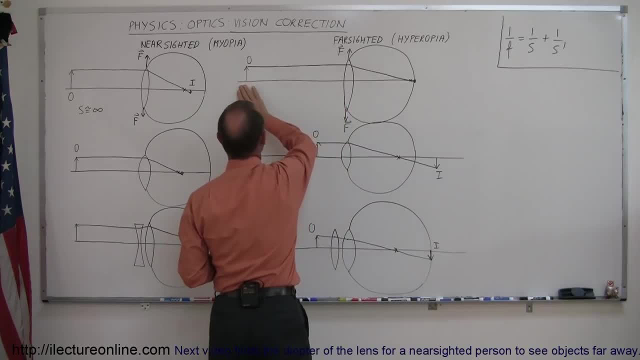 A far-sighted person has no problem looking at objects that are really far away, because the lens is shaped in such a way, and the eyeball is shaped in such a way, that when the muscles pull on the lens and the lens gets made thinner, the focal point falls far enough back, so then an image is formed right there. 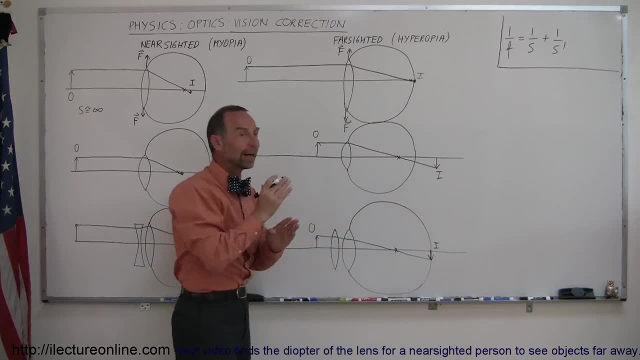 The image is formed which is right past the focal point and right on the retina. so no problems for people that are far-sighted to see things far clearly. But then what happens is when you bring the object closer, Then of course the muscles will let go. the lens begins to shape more like this. that brings the focal point in. but if the lens doesn't bulge up enough- and of course there's no muscles that make the lens bulge up, the lens bulges by itself if the muscles don't stretch it. 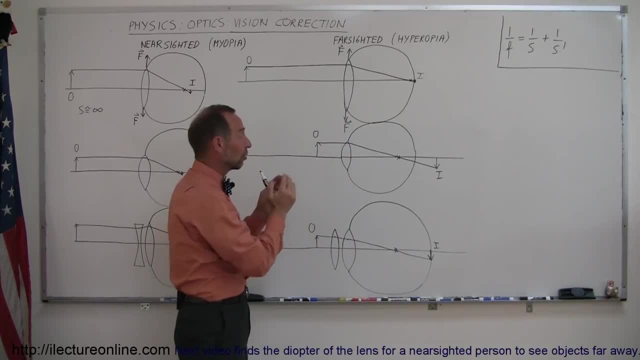 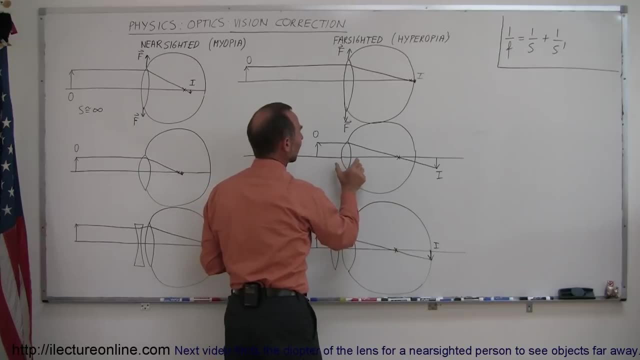 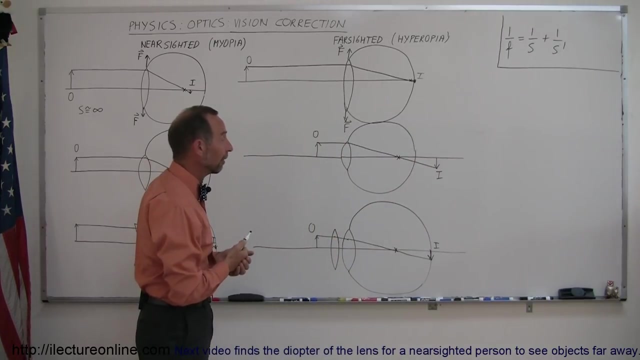 Now, as people get older, the lens doesn't quite get back to its normal shape, in a more bold shape, when- because like they were when they were younger, which means that the focal point doesn't get pulled to the left enough, which means that the image, And therefore that image will look very fuzzy, will not look clear or crisp. 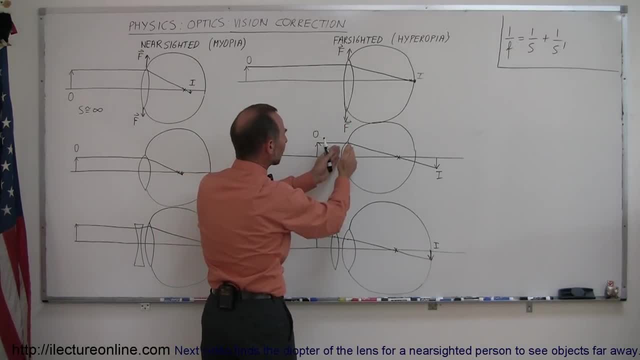 So the only way to do that, since the muscles, when they relax, don't allow the lens to move to the right or bulge up enough, as I should say, Then we need some help to make that happen. So a second converging lens in front of the eyeball lens will cause the focal point to move further ahead. 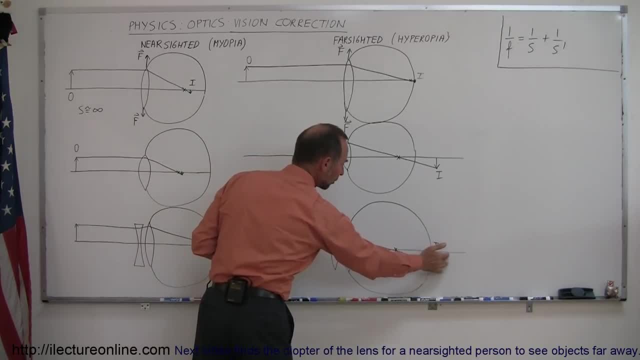 I've changed the focal quality levels later on because I didn't want the focus to be on either side. Now there's no till. if it doesn't look like, it should be satisfy. Hopefully further to the left, which will bring the image into the left as well. 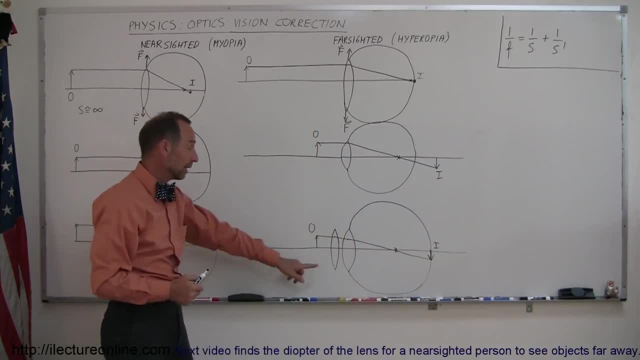 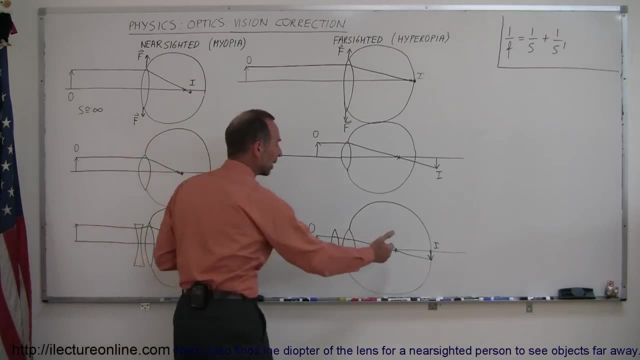 which then will fall right on the retina and then you'll see clearly. These are then called reading glasses, lenses of reading glasses. They're converging glasses. It's kind of like a magnifying glass. It simply brings the image in closer and you can then see things clearly. 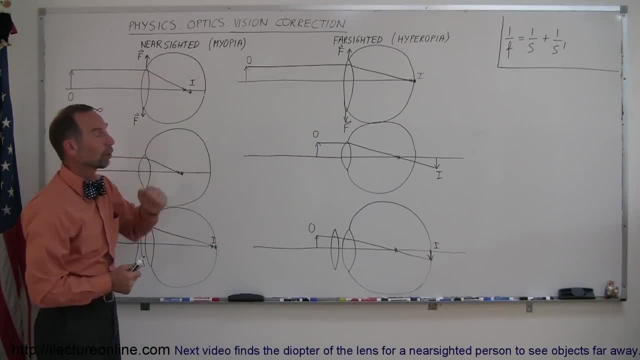 And that's how we correct vision, either if you are nearsighted or you're farsighted. And so the next several videos, we'll actually do some practical things. We'll actually, depending upon the eyesight, figure out what kind of lens you need. 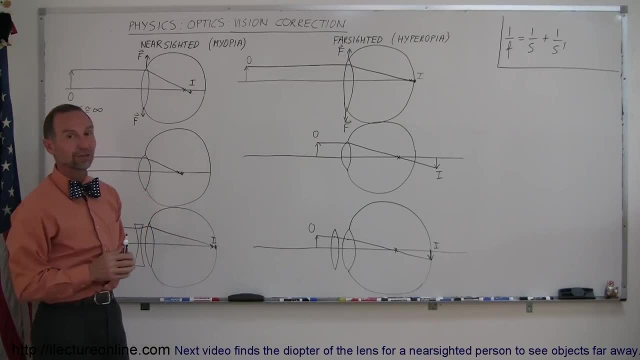 in order to see clearly if you're either farsighted or if you're nearsighted. That's next.